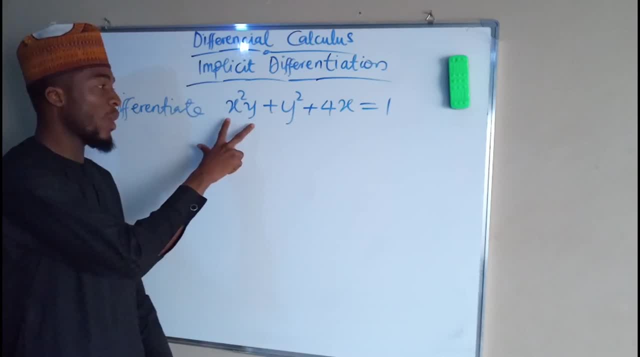 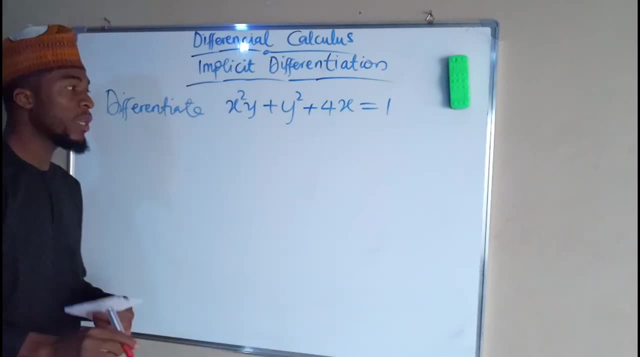 But the first term is x squared y, Meaning we are going to apply product rule here. We are going to differentiate this one independently and this one the last time. So product rule says you keep one of the terms constant and differentiate the other. 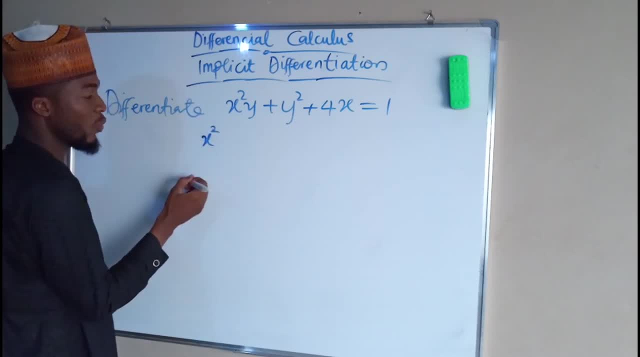 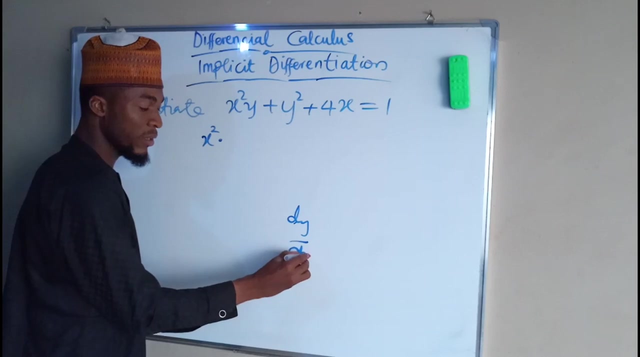 So now, if I keep x squared constant, I now want to differentiate y, So I am going to differentiate y. If you differentiate y, you are going to obtain one. But remember, the derivative of y is always expressed either dy over dx, y' or f of x'. 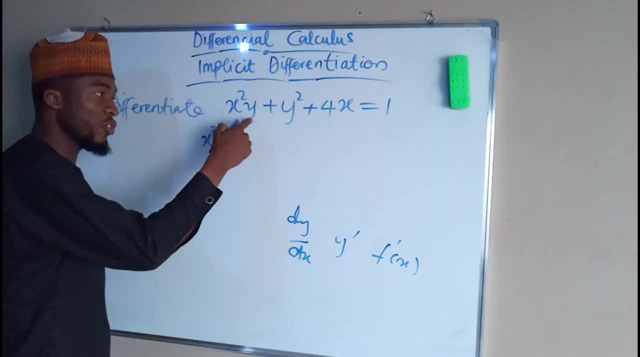 So you can use either of them. First of all, we need to differentiate the function y, which is 1.. Then you multiply by either of these three. So let me apply y', which is the same thing as dy over dx. 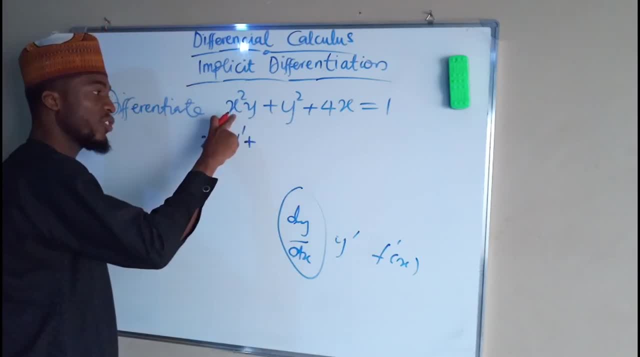 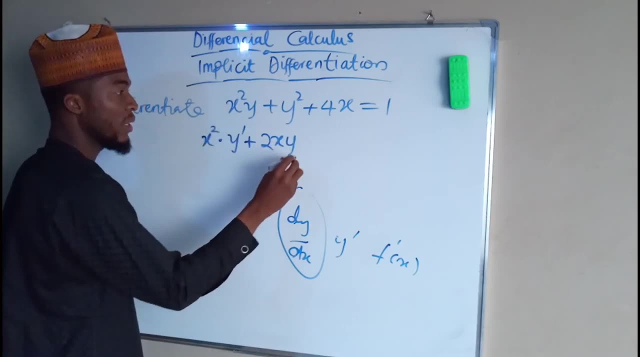 Plus. I now want to keep y constant and differentiate x. If you differentiate x, you are going to get 2x. Then y is constant, Then plus. This time, if you differentiate it, you are going to obtain 2y. 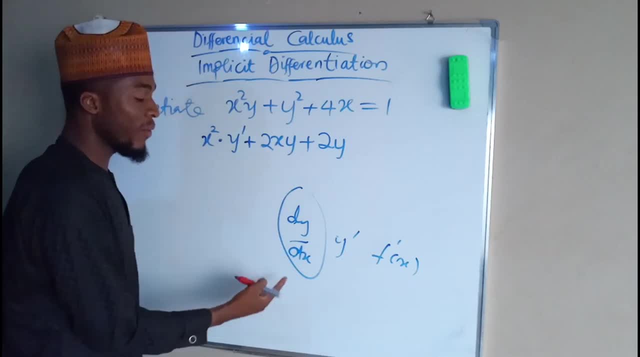 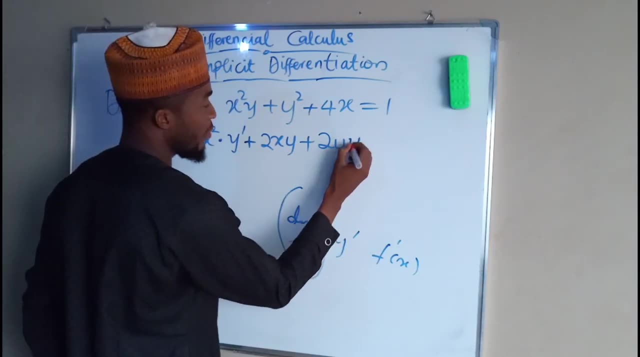 But I told you, once you differentiate y, you have to multiply by either dy over dx y' or f of x' So I have my y' here, Plus, If you differentiate 4x, you are going to obtain 4.. 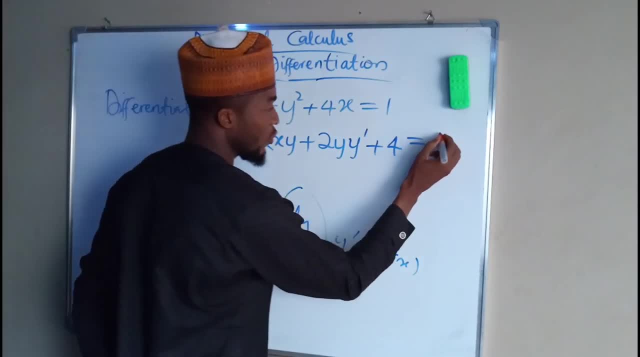 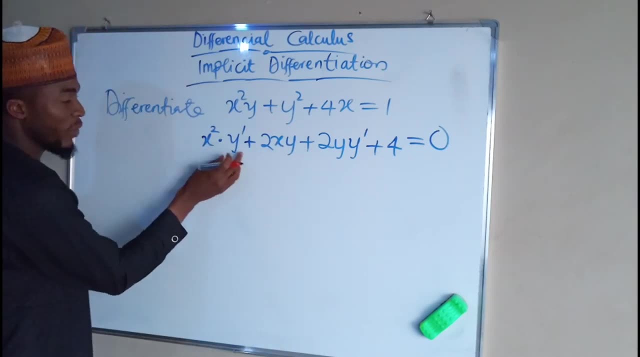 Because the derivative of constant time is 0. So we have 0 here. Now I want to collect like times, Thus with y' together. So here I have x squared times y', which is x squared y'. 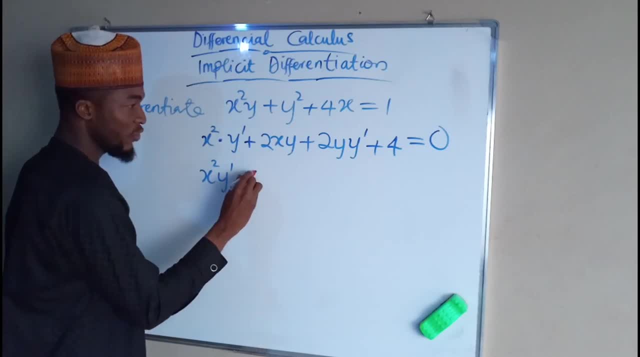 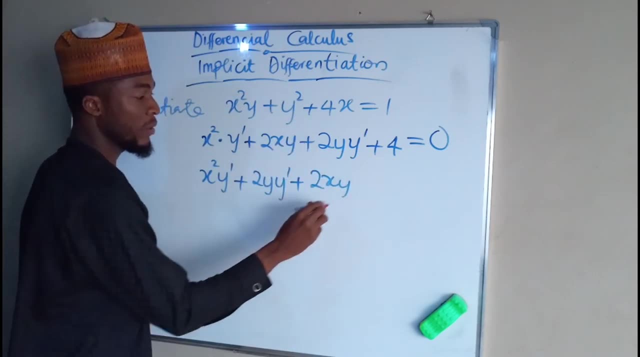 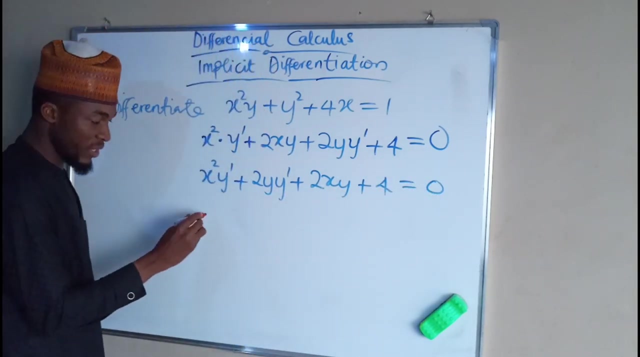 Then I will bring this one to this place, which is 2y, y' Plus 2xy plus 4.. Because 0. By factorization I will have y' out. Then inside the bracket I will have x squared plus 2y. 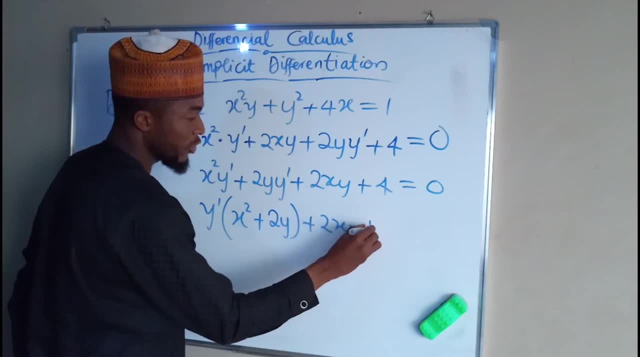 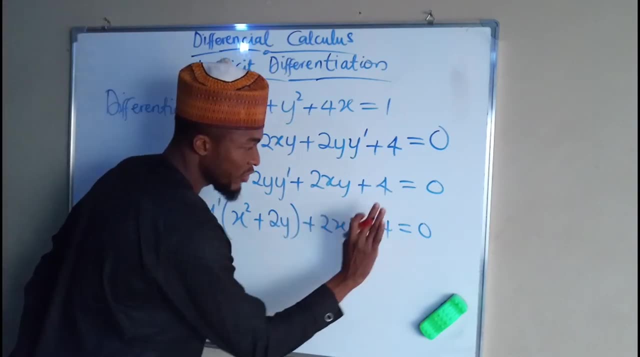 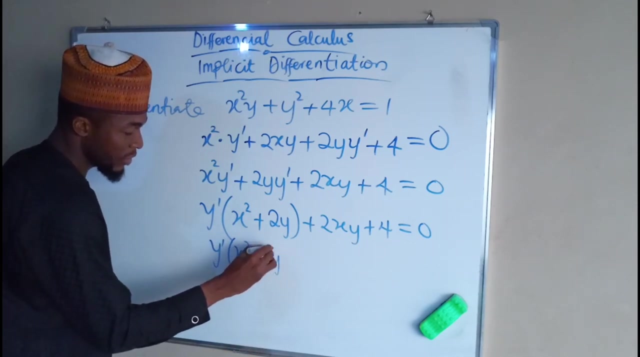 Plus 2xy plus 4.. Because 0. Then now I want to take all of these two times to the right hand side, leaving these times So y' x squared plus 2y Will be equal to. 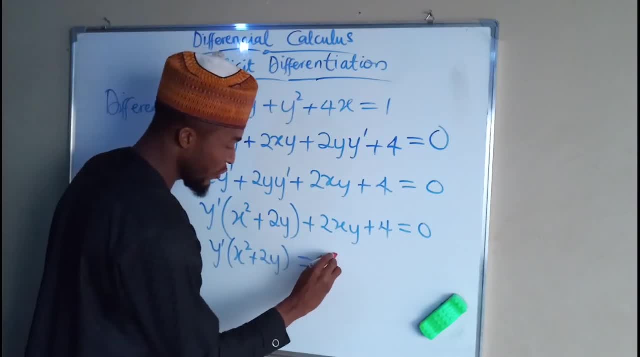 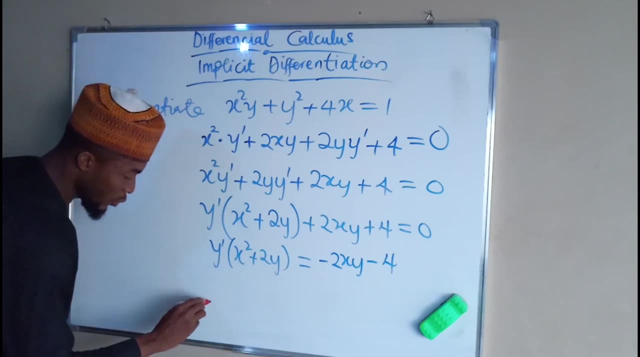 If this term crosses equality sign, it turns to negative 2xy. The other term will change to negative 2.. Now to find y' which is dy over dx. you can write it as dy over dx. Then you say: x squared plus 2y. 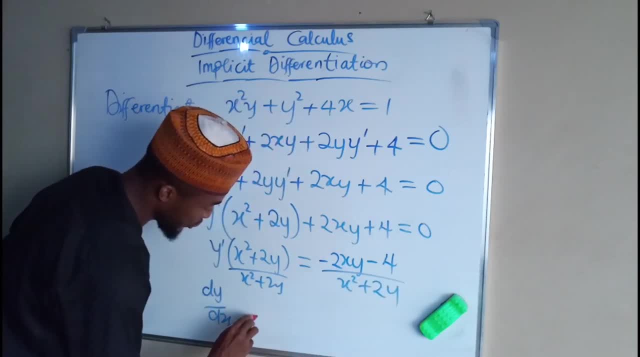 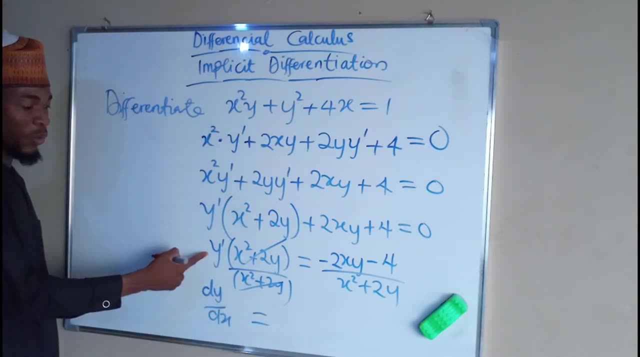 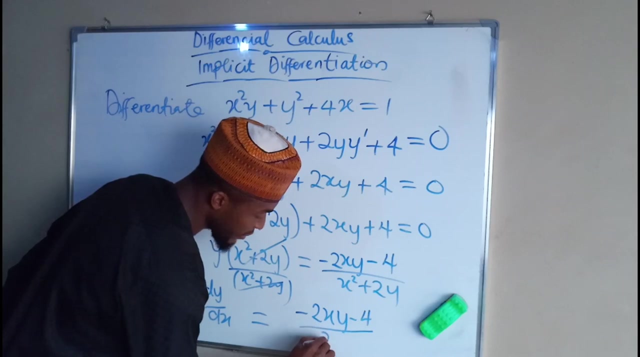 x squared plus 2y, Which will give us This will cancel this, definitely, Leaving only dy over dx, Which is the same thing as y' equals minus 2xy minus 4 divided by x squared plus 2y. This is the derivative of this implicit function. 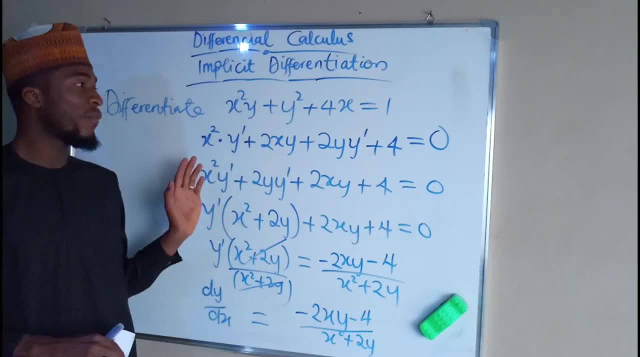 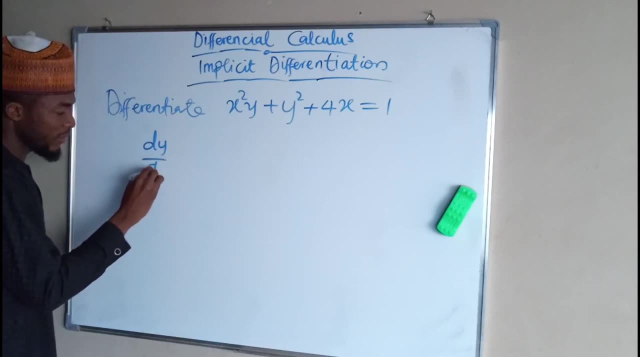 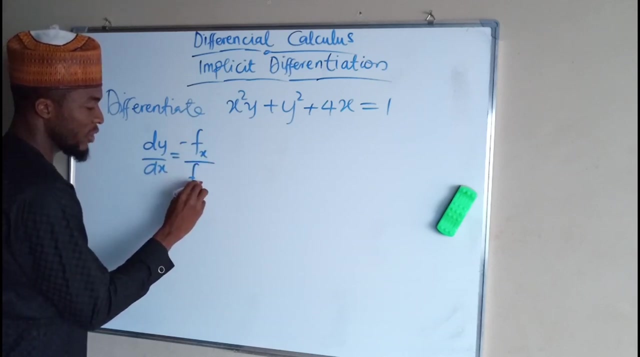 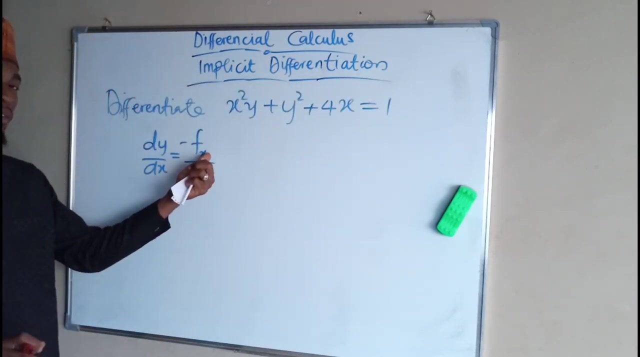 Now I want to apply the particular formula used in finding the derivative of an implicit function. dy over dx is equal to f minus f subscript x. This means we are going to differentiate the whole of the function with respect to x alone. Whatever we get, we multiply it with negative. 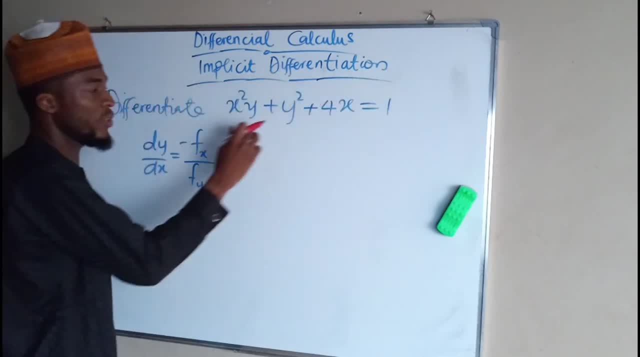 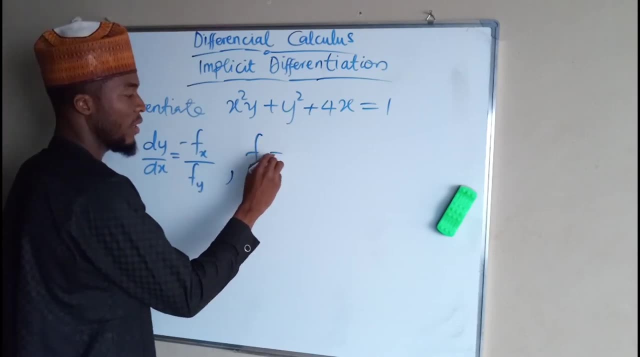 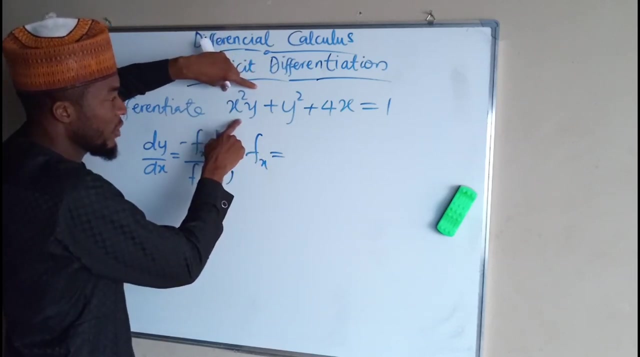 Then we divide by the derivative of the function with respect to y alone. Let us differentiate the function with respect to x, which is f subscript x. This will give us This term has x. We are going to differentiate this term With respect to x alone. 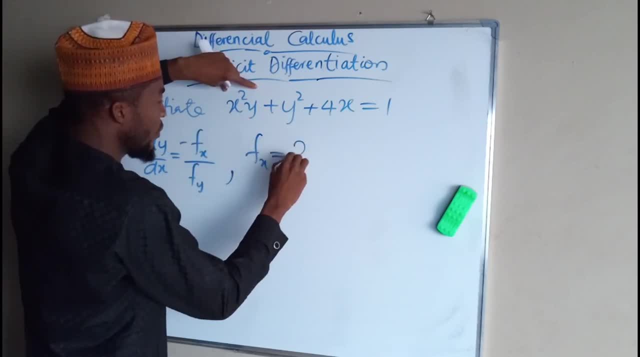 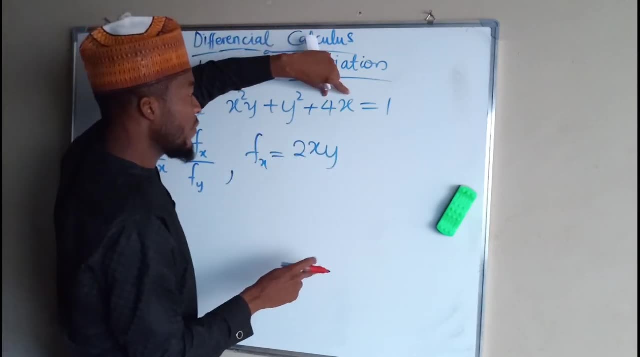 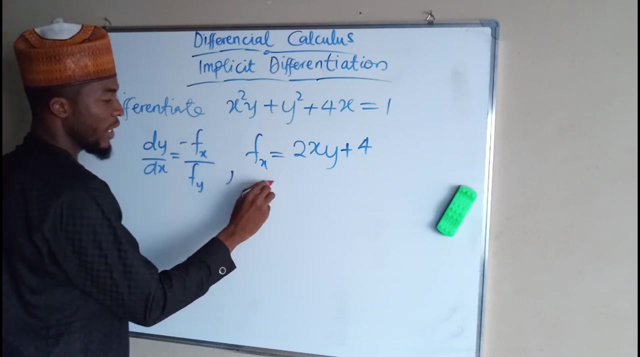 Given y constant, So this will give us 2xy. Forget about this, because we have no x here. Then you differentiate this, Which will give us only 4.. Remember, we are going to multiply with negative, So this will give us minus 2xy, minus 4.. 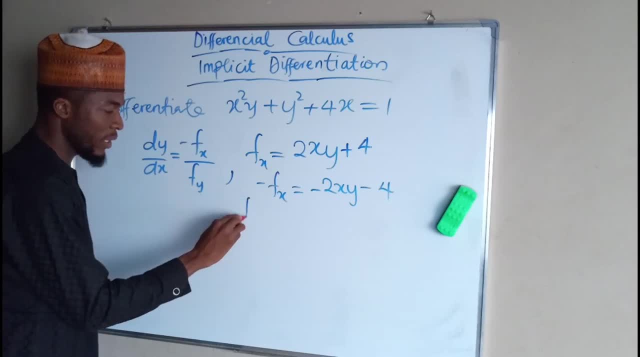 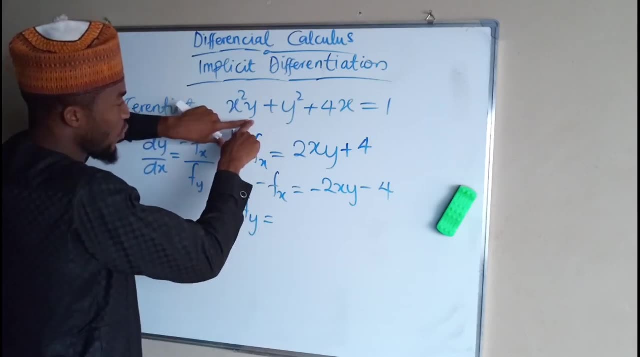 Then the second one, f subscript y. This will give us minus 2xy, minus 4.. We are going to differentiate the whole of the function with respect to y, The first term. if we differentiate y, we are going to obtain only x squared.